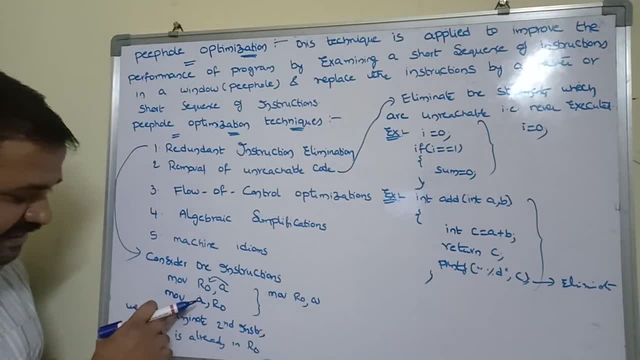 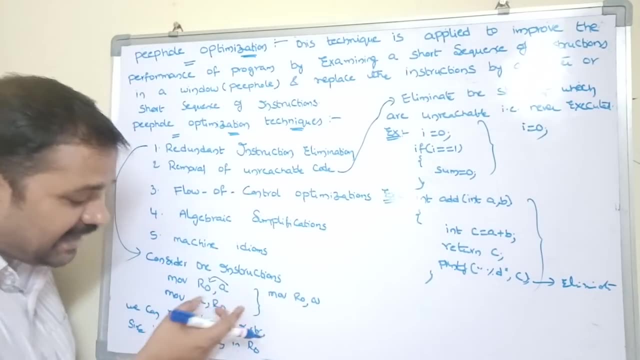 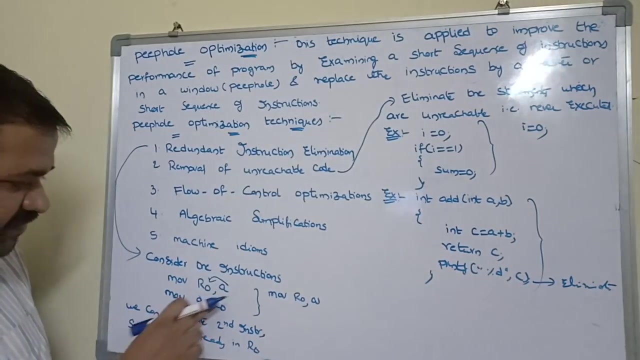 Now or not contains a value. So in the second instruction what we are doing Once again we are moving or not value to a, But or not already contains a. So there is no need to execute the second instruction. If we execute the second instruction, even though then the result of a or or not won't change us, So we can eliminate the second instruction. Why? because since a is already in or not, 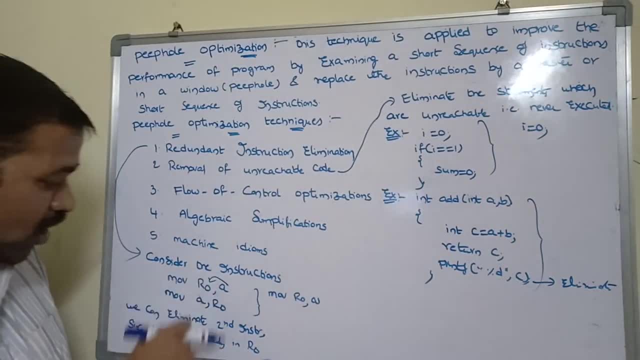 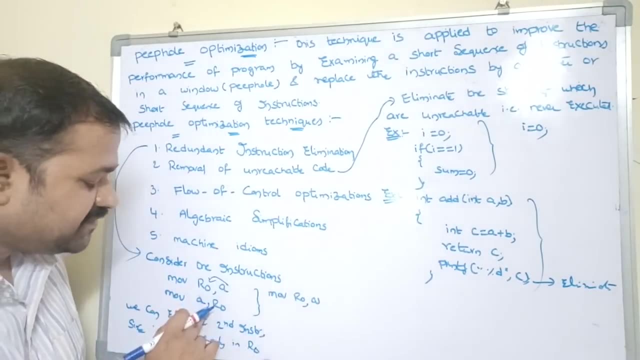 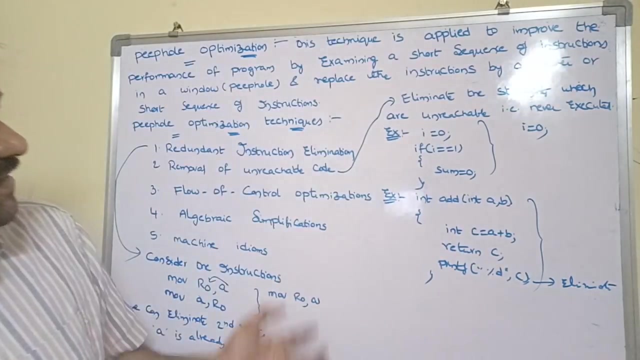 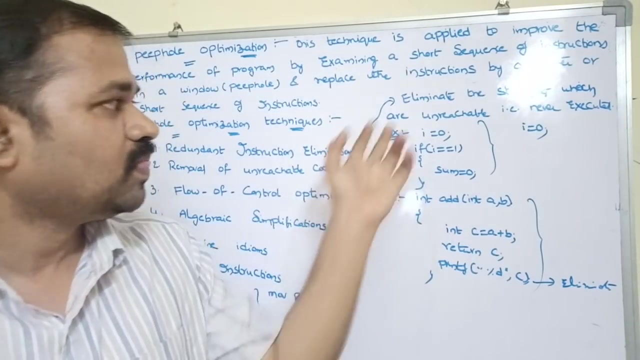 A value is already available in or not. So, after optimization, what is the code? We can have only the first statement. Move or not comma a. We can eliminate this statement Why? because already a value is available in or not. Now let's see the second one. The second technique is removal of unreachable code. So remove the statements which are unreachable. So unreachable means never executed. 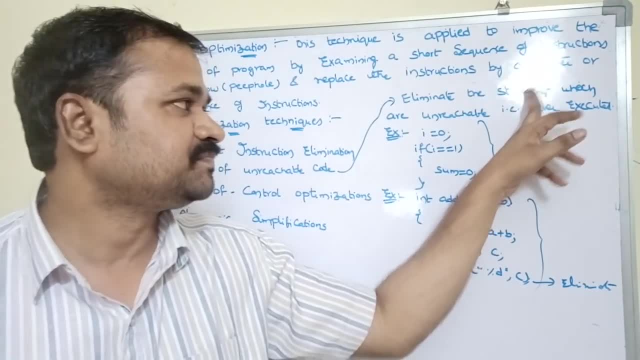 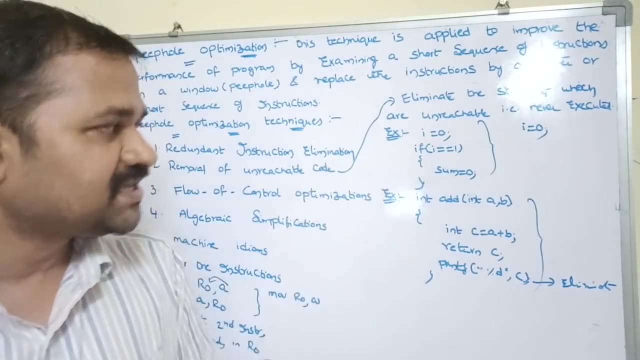 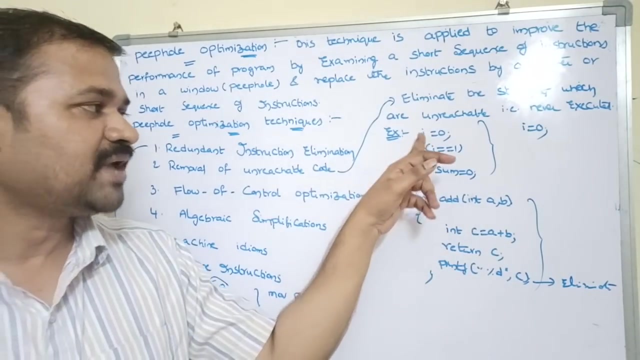 So eliminate The statements Which are unreachable. So unreachable means never executed statements. Let's take two examples here. i is equal to zero. If i double is equal to one, Then execute some value, So i is initialized into zero. So what will happen now? 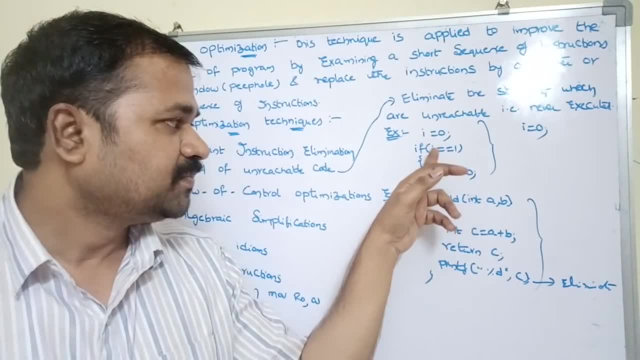 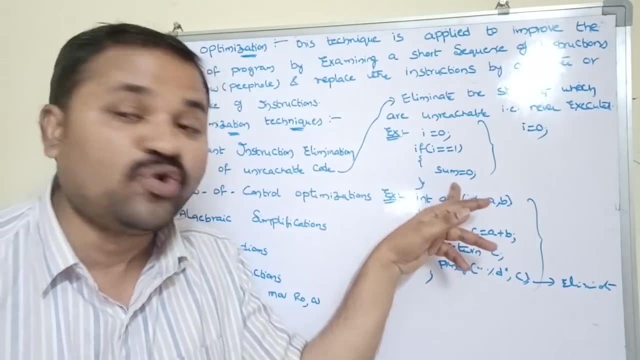 Throughout the program. i value should be zero only. But here, what is the condition? Zero double is equal to one, So this condition is false, So this body won't execute. why? because every time this condition will be false, audit so we can eliminate this block. 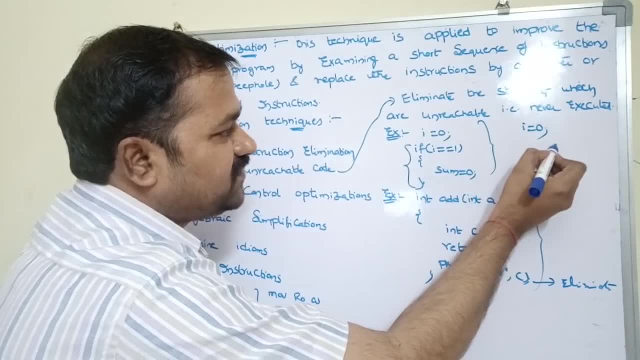 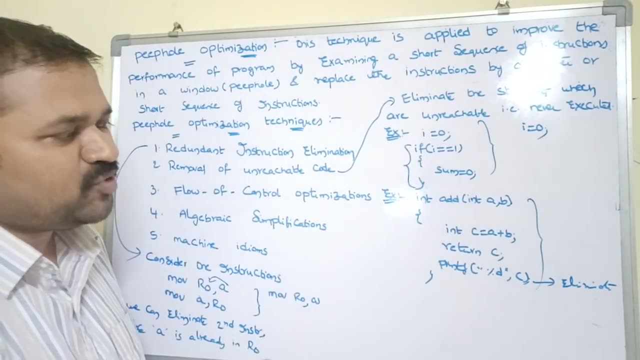 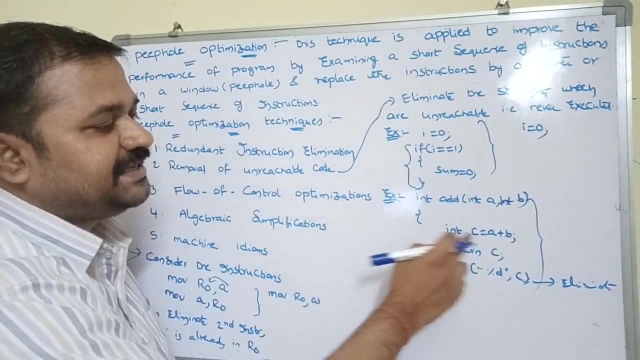 so, after optimization, what is the code here? i is equal to 0, so this is nothing but unoptimized code. this one is nothing but optimized record. let's take one more example: int add of int a comma, int a comma, int b. next, int c is equal to a plus b. return c: print of percentage d comma c. so with: 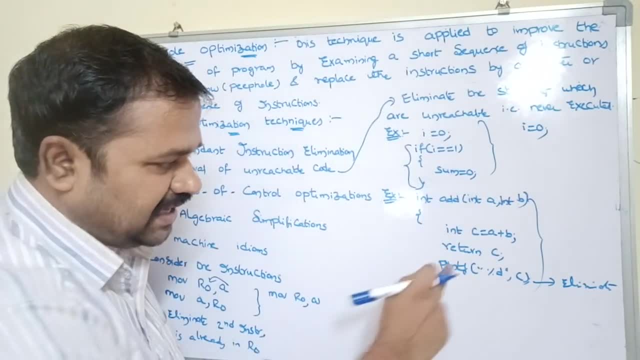 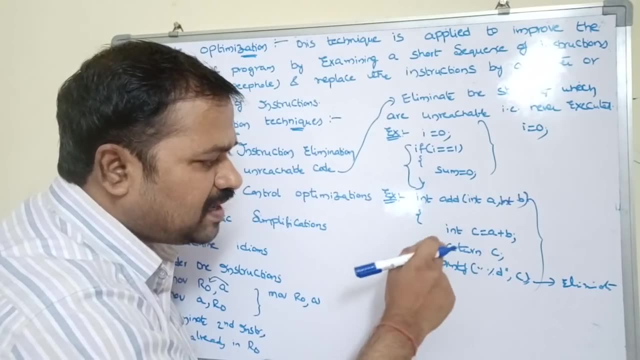 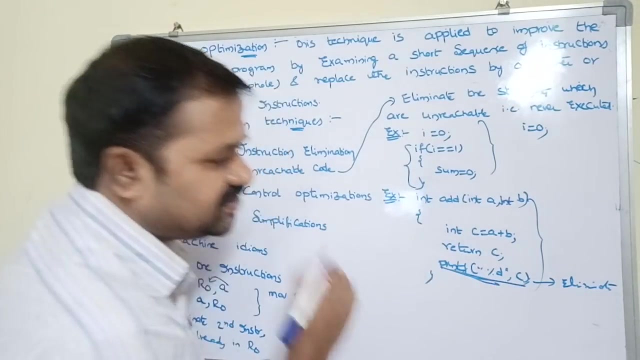 the help of add function we are adding two integer values and we are returning that value. so whenever written statement is executed then it returns a value from this called function to the calling function. so print of percentage d, comma c. so the statement never executes. so we can eliminate this. 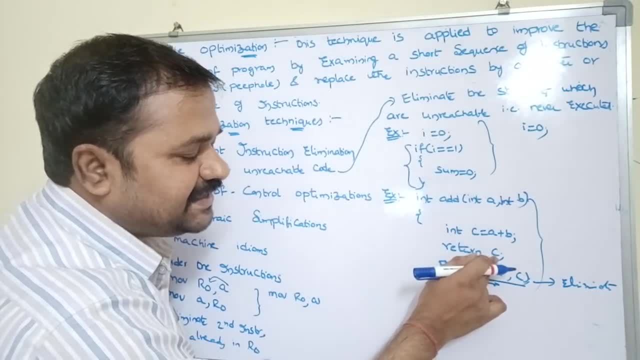 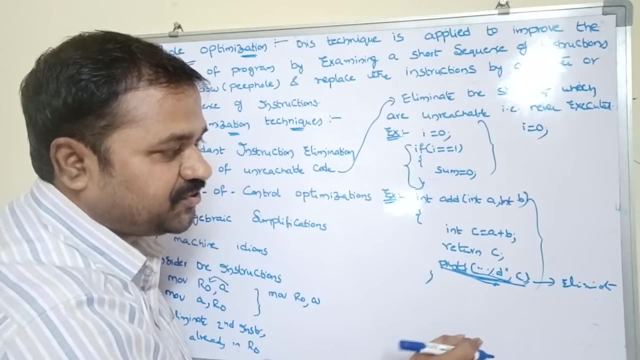 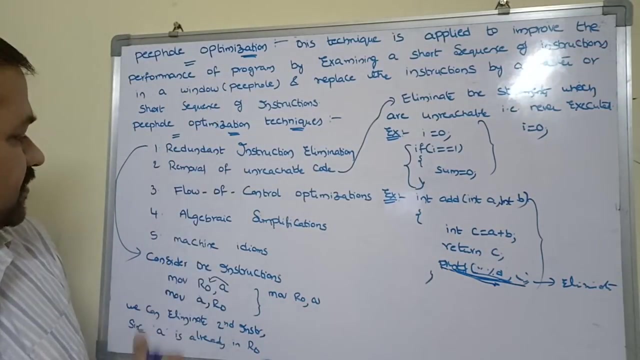 statement, because once written is executed, then it returns c value from called function to the calling function, so c value won't print it. so this is nothing but an optimized record. so what is optimized record, optimized report, is nothing but eliminate this print of statement. now let's see. 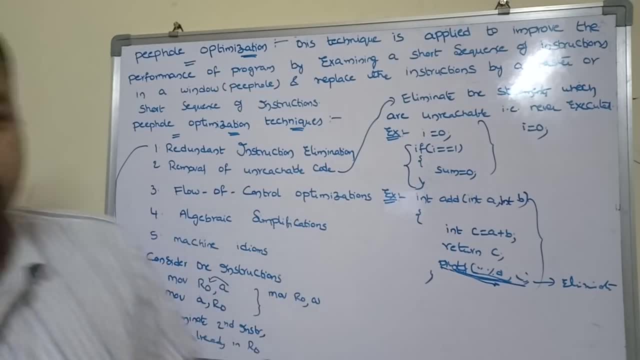 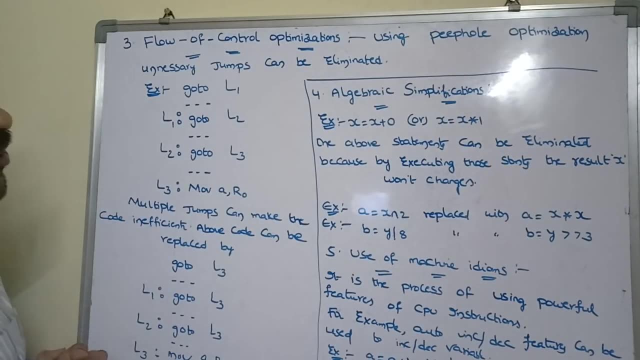 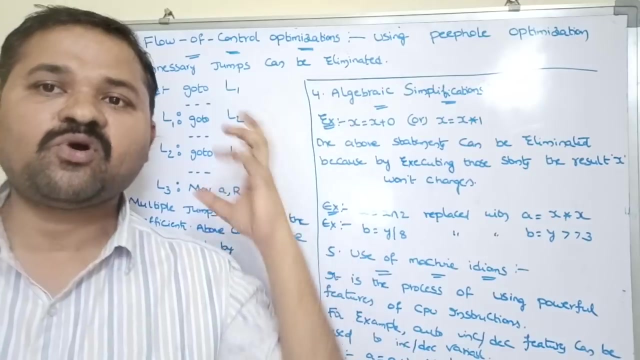 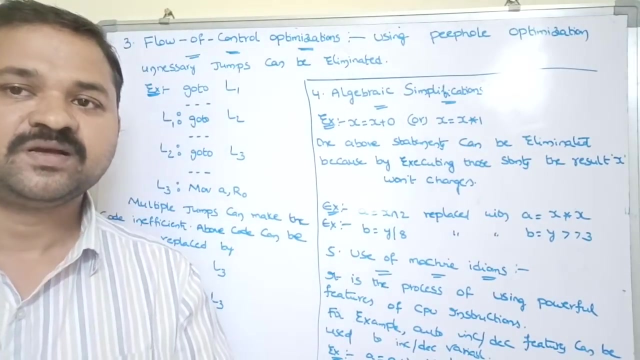 the third, four and, yeah, fifth techniques. now let's see the third approach: flow of control optimizations using people optimization. so flow of control means the control will be transferred from one place of the program to another place of the program. so by using people optimization we can eliminate unnecessary jumps. 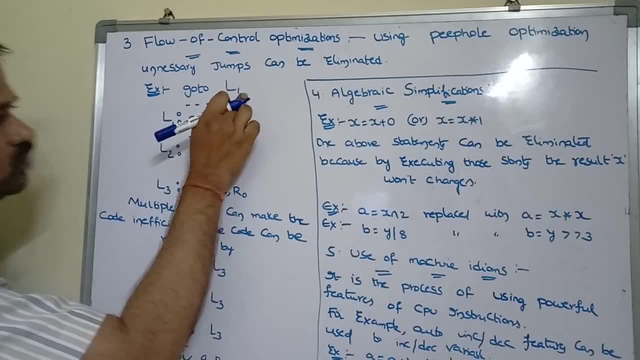 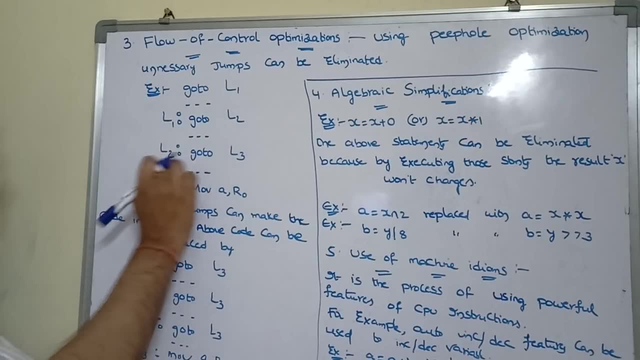 if you take this example, go to l1, so we go to the label l1. next go to l2, so we go to the label here too. so these are the number, some statements. next go to l3, so we go to the label here, 3.. so in. 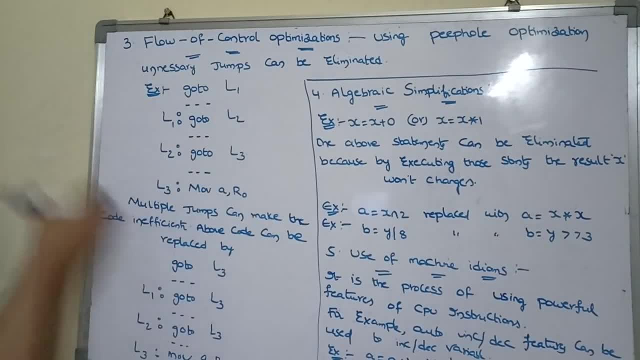 have some statements. so instead of moving from one label to another label- because here the destination label should be l3 only so directly we can go to l3 instead of l1. so we can, we can eliminate these multiple jumps like this. so go to l3, so directly we can go to l3. now l3, so this is. 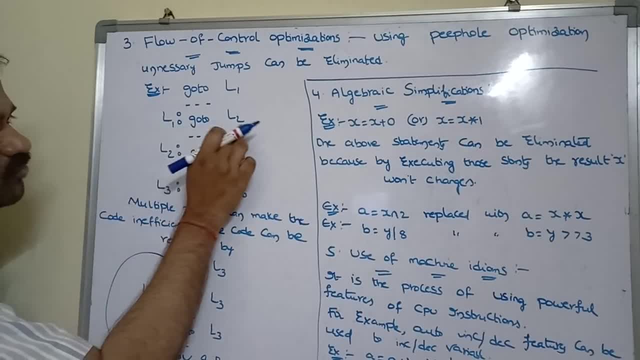 the statement here: next: l1 from l1 we have to go to l2. next, from l2 we have to go to l3. so instead of going like this: from l1 directly we can go to l3. so l1, so go to l3, so directly we can go to l3. 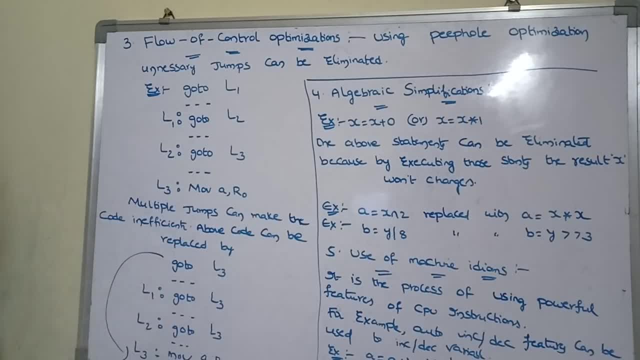 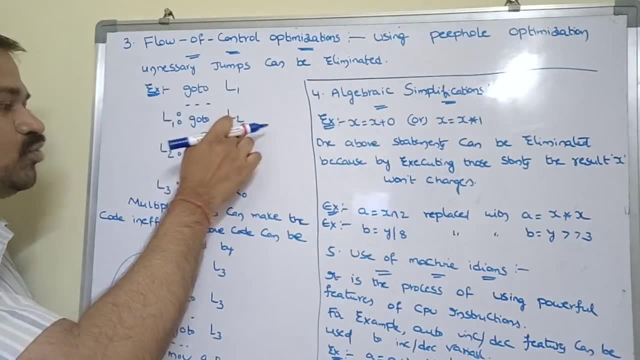 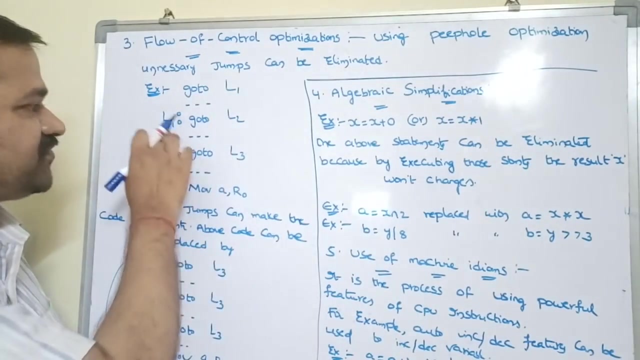 likewise, from l2, also directly, we can go to l3. so likewise we can eliminate the multiple jumps. okay, so instead of moving from l1 to l2, l2 to l3 directly, we can go from this directly. we can go to l3. so likewise from l1 also. instead of going to l2 directly, we can go from l1 to l3. 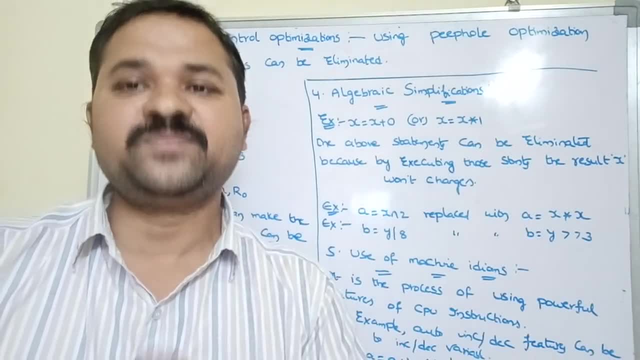 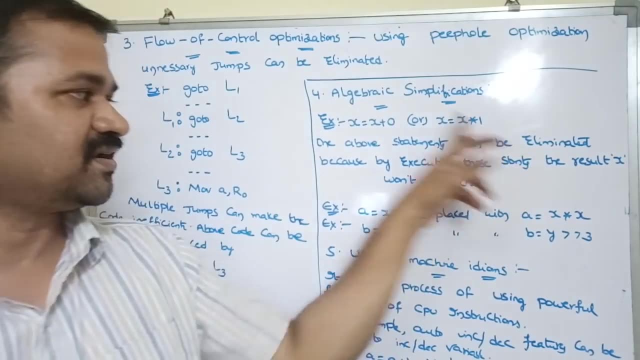 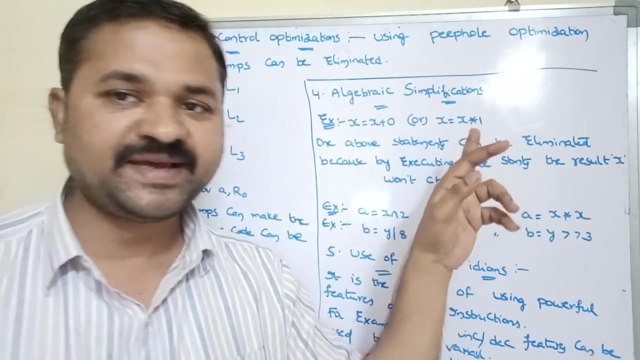 directly. and the fourth one is algebraic simplifications. let we have an expression like this: x is equal to x plus 0, or x is equal to x in x, star 1. so x is equal to x plus 0 is nothing but x only. x is equal to x star 1 is nothing but x only. so by executing these, 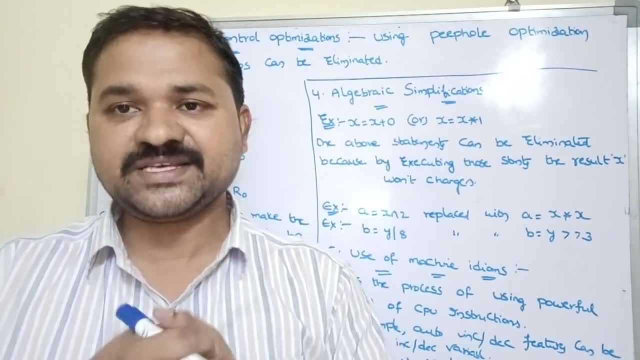 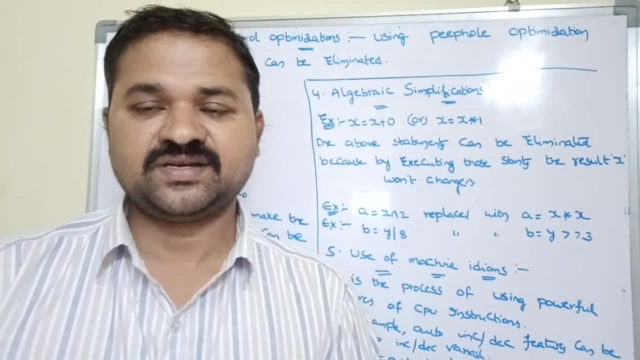 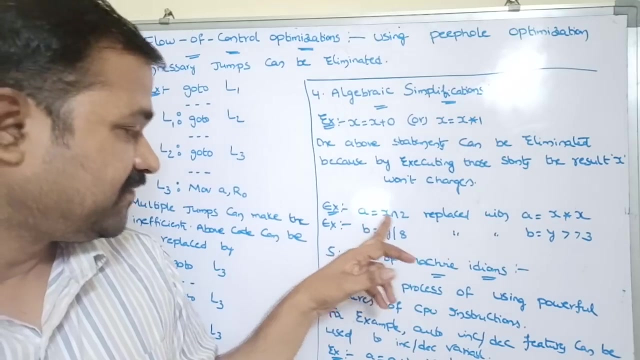 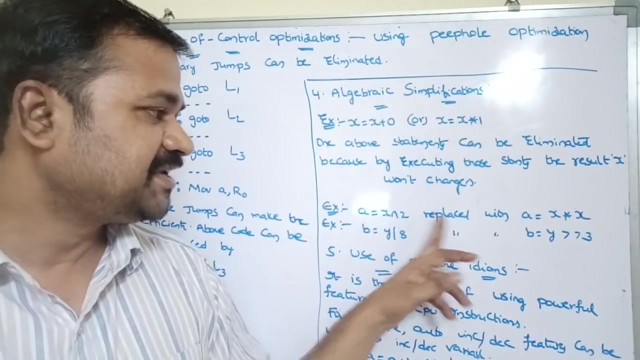 statements: the result of x won't changes, so it is not necessary to execute these instructions here. we can apply reduction strength also, so strength reduction. so that means we have to replace the expensive operator with the cheapest operator. okay, let we have an operator like this: a is equal to x, power 2: this statement. this is nothing but power operator. this statement. 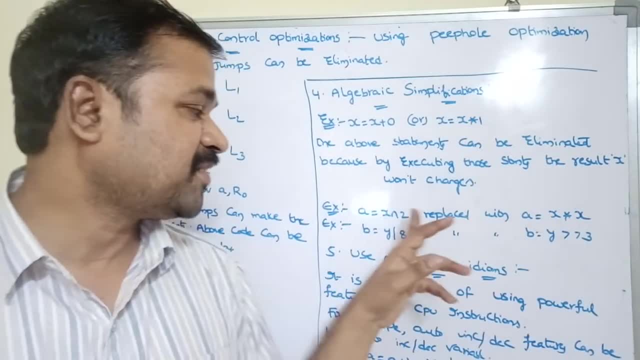 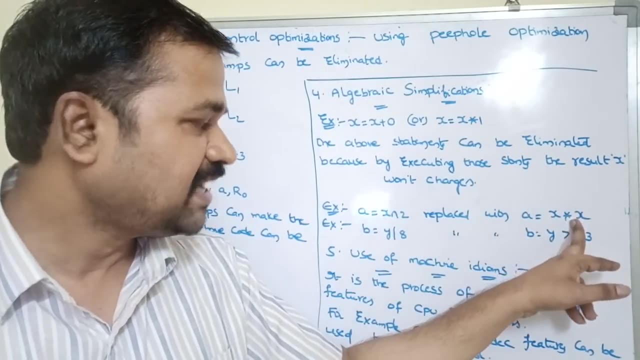 can be replaced with a is equal to x, star x. why? because power is nothing but expensive operator, whereas star is nothing but cheaper operator. okay, so we are replacing power with multiplication operator. next, b is equal to y division 8. so here division is an expensive operator. 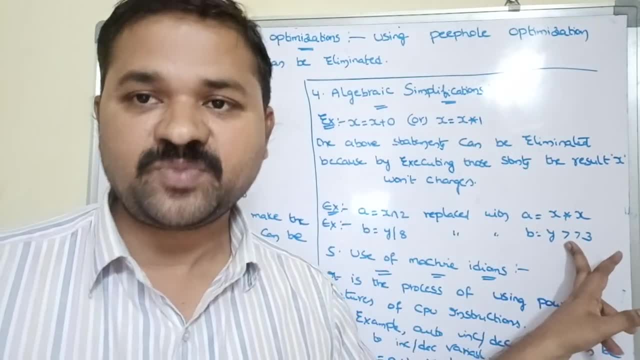 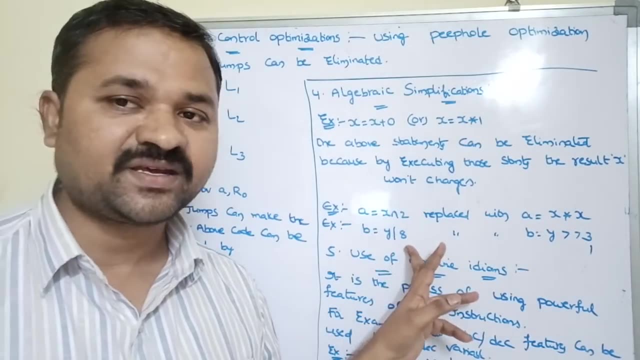 here, in order to perform this operation, we are using right shift operator. we know, if you right shift one operator, then the result is division of two. but here what is the result by eight? so by eight means we have to move uh, three positions to the right side. okay, 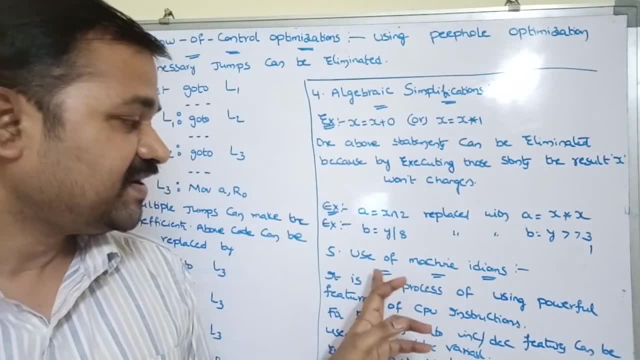 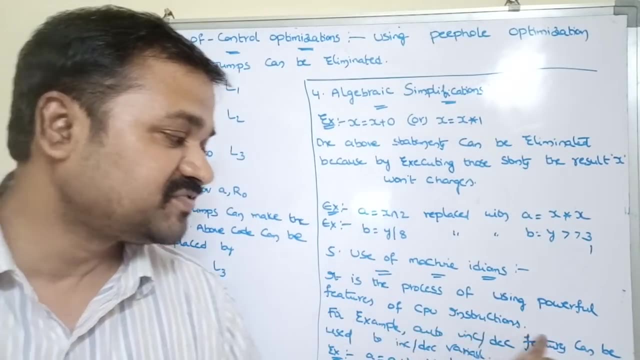 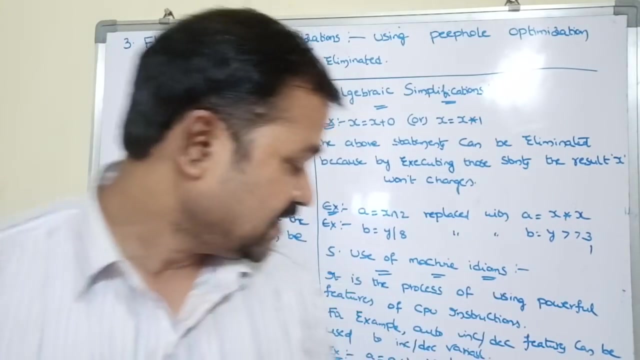 so this is nothing but algebraic simplifications. and the last one is use of machine idms. here we can. it is the process of using powerful features of cpu instructions. so here, in order to perform the operations, we can directly use this cpu instructions. if you want to perform an addition operation, we may use an instruction like this: a is equal. 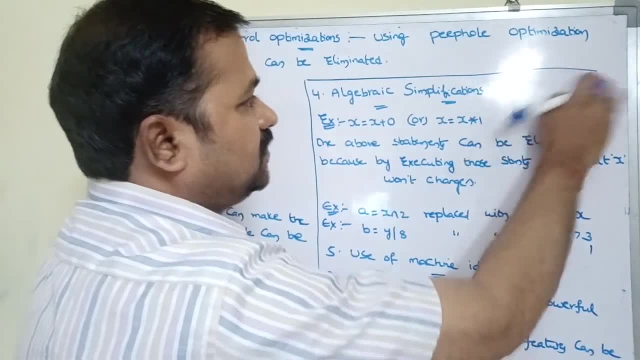 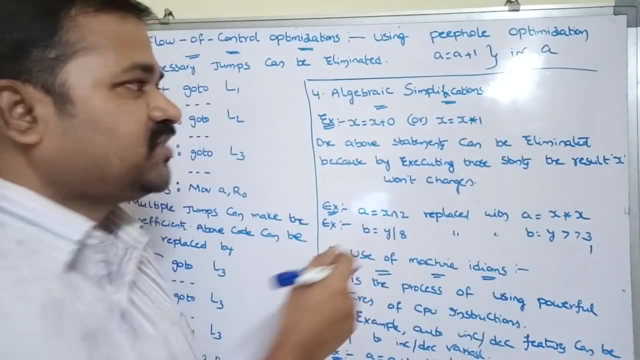 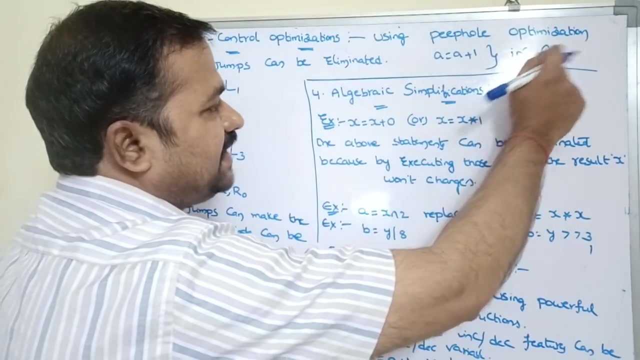 to a plus one. a is equal to a less than so a is equal to a plus one, so this statement can be replaced with increment here. so increment a is also nothing, but a is equal to a plus 1. okay, so instead of writing this one, it is better to write i n c? a. 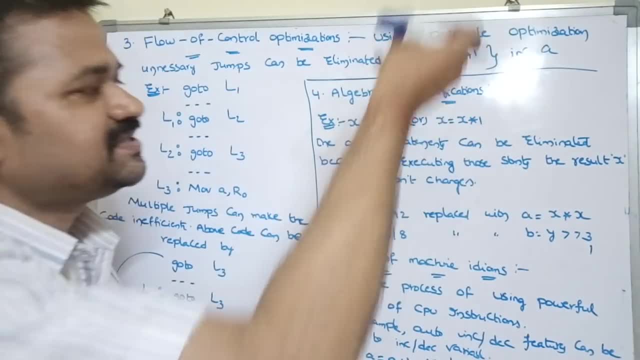 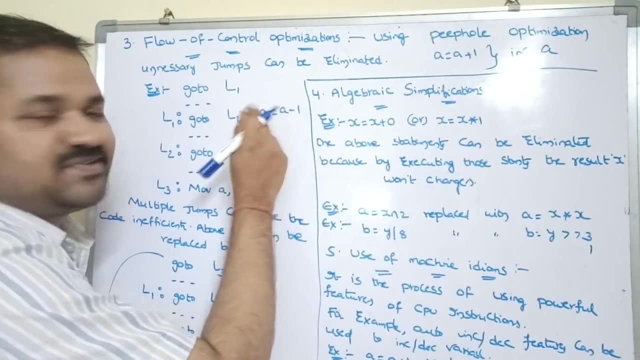 Why? Because it is CPU instruction. it executes the data in a faster manner. Let us assume that we want to perform some decrement operation, So we can write the instruction as: a is equal to a minus 1. So this statement can be replaced with decrement a. this statement can be replaced with decrement. a, because decrement is nothing but some CPU instruction. It performs the operation in a faster manner. So this is about the whole optimization.